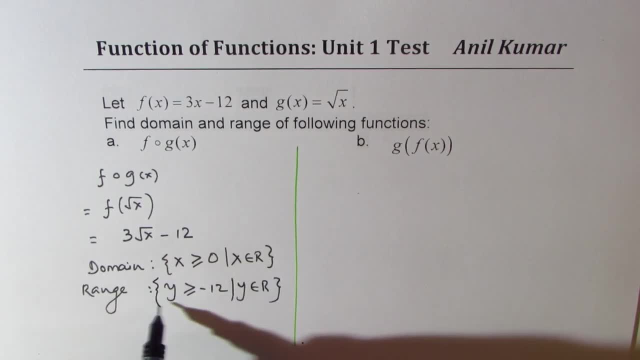 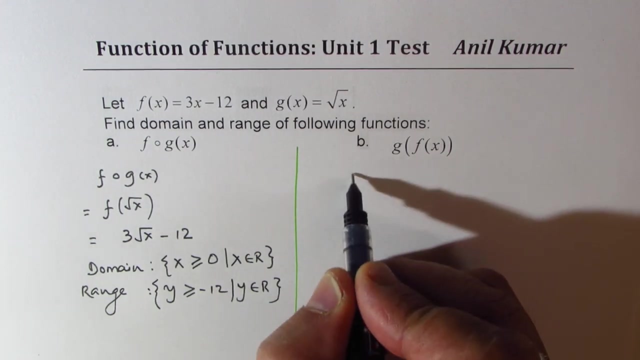 where y belongs to real numbers. so this set of these numbers. so that is how you get domain of range of f of g of x. now you can actually pause the video, find the function g of f of x and write its domain range. so let's do it now. g of f of x is equals: 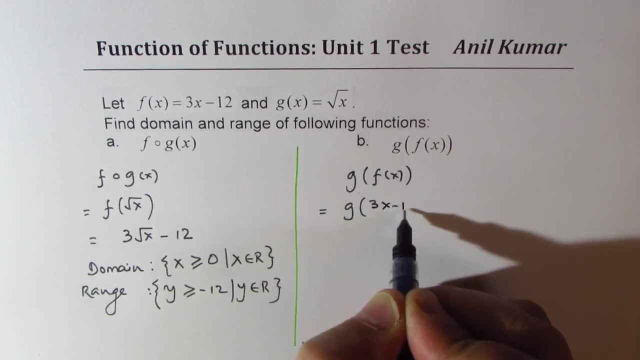 to g of f, of x is 3x minus 12, which is square root of 3x minus 12. now, in this case, we told, ofunciating that the domain with zero in it, you need a domain withinarea. Similarly, what you could do is you could actually: 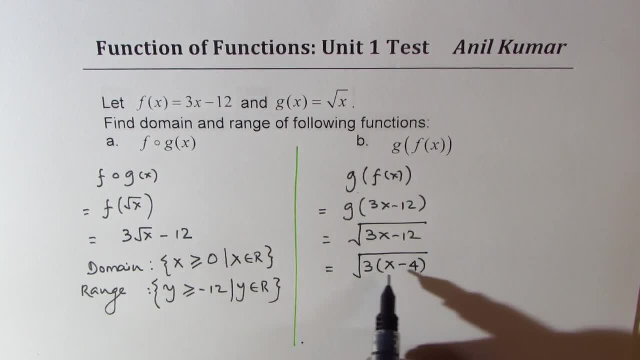 factor ourselves, so we get x minus 4. now with this, and if you think about this, what you could do is you could actually factor out three, so we get X minus 4. now that gives you that the domain here is x is greater than equal to four, where X belongs to real numbers and the range is 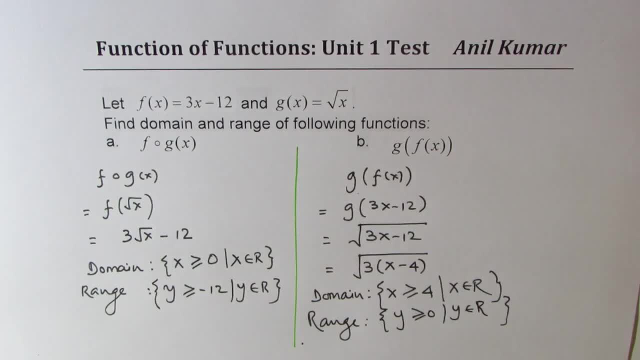 y is greater than equal to zero, where y belongs to real numbers. so it's kind of better to really solve this point and figure out them already, and you have to figure them out. so what you can do is останов according order in h a. It doesn't really take much time, but make sure that you get the right answer. 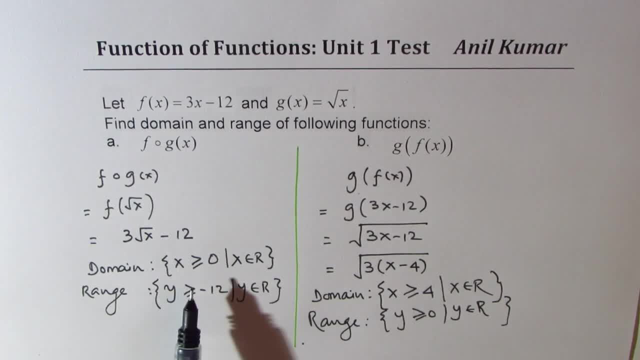 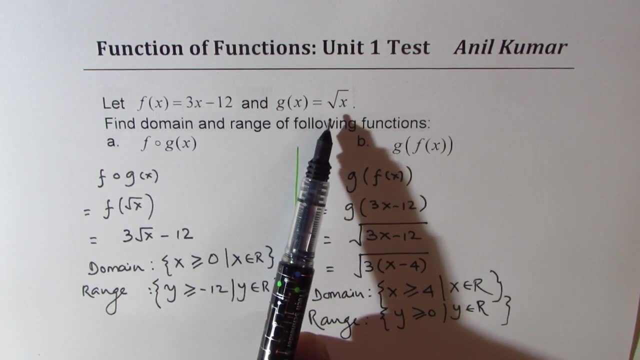 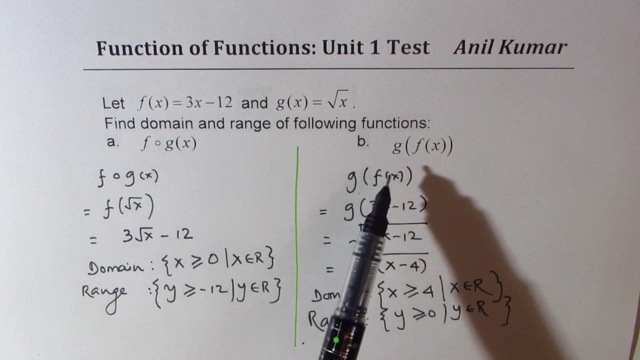 Correct. So what you notice here is that the domain Actually is restricted because of the function square root of x. Okay now here, Square root of x has to be greater than equal to 0, but when you do g of f of x, f of x comes in the. 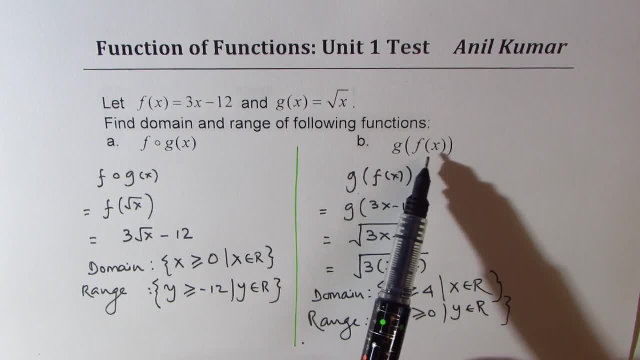 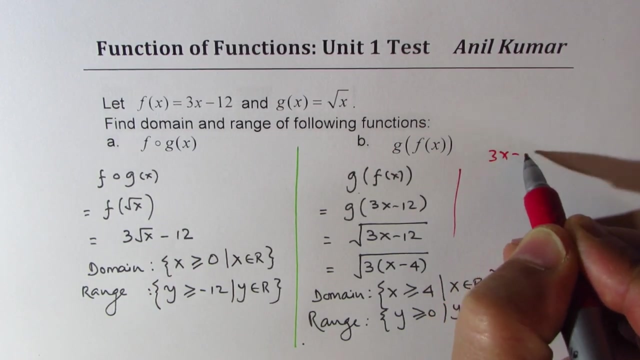 Inside function. so we are looking into range of f, of x, which should be positive. You see that. so that gives you x greater than equal to 4, right? so in this case We are looking for the range 3x Minus 12 to be greater than equal to 0, so that gives you 3x is greater than equal to 12. 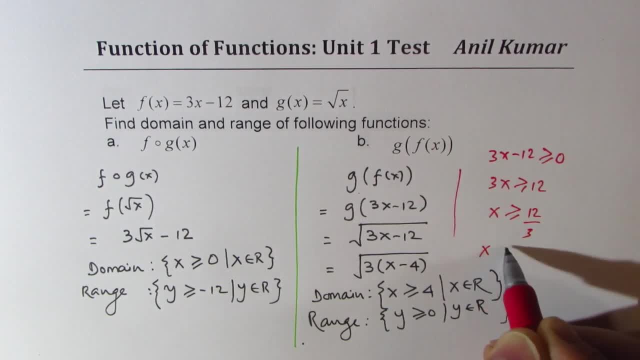 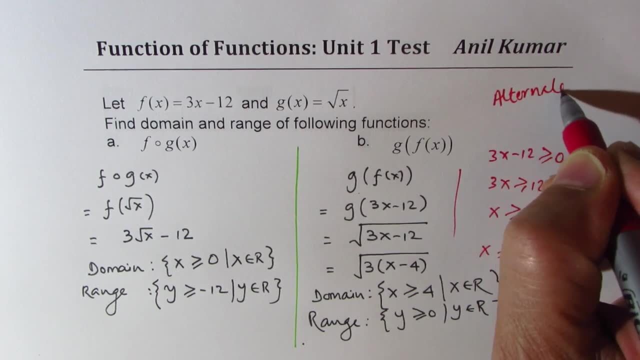 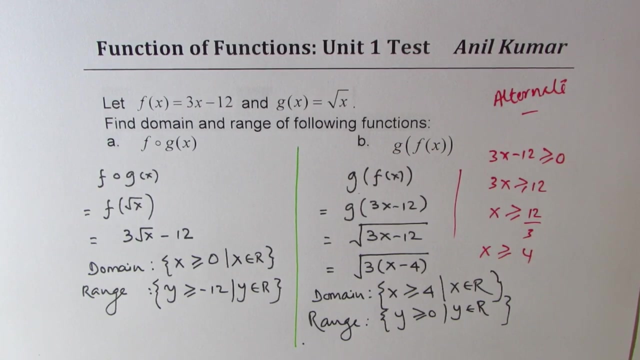 X is greater than equal to 12 over 3. so x is greater than equal to 4. so that could be the alternate method of solving Without finding functional function. that's what I'm trying to see, right? so that is how you could actually do it.